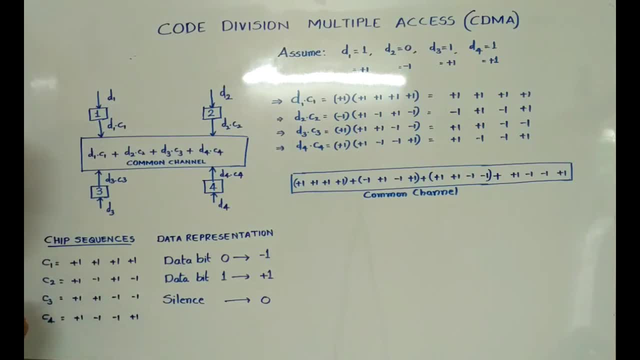 And this sequence like this is the coding action. This is also called orthogonal sequence. What is this orthogonal sequence? Okay, So the speciality of orthogonal sequence is If you multiply C1 with C2, you will get 0.. C1 with any other one, like if you multiply any code with other code, you will get 0. 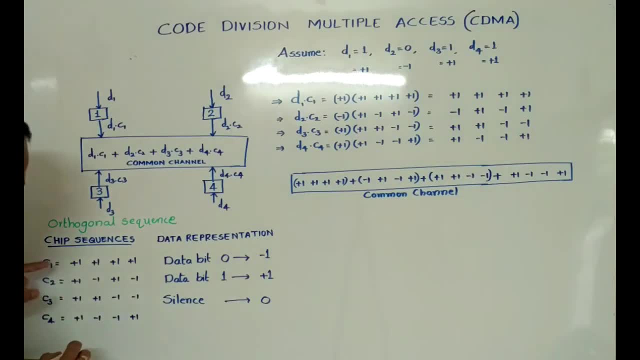 For example, I am taking this. For example, I am taking C1 and C2, I will multiply both Plus 1 into plus 1, plus 1.. Plus Plus 1 into minus 1, minus 1.. 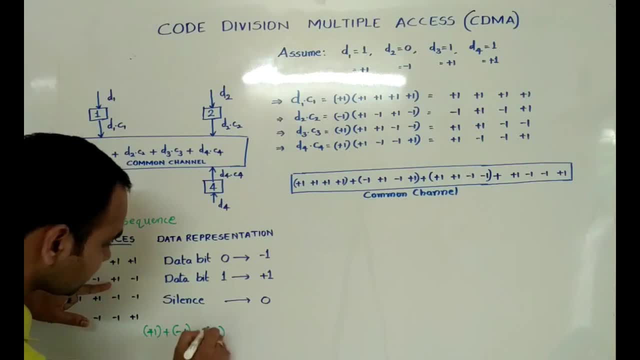 Plus Plus 1 into plus 1, plus 1.. Plus Plus 1 into minus 1, minus 1.. So if I add this, what happens is you will get 0. And if you multiply, this is the same code. 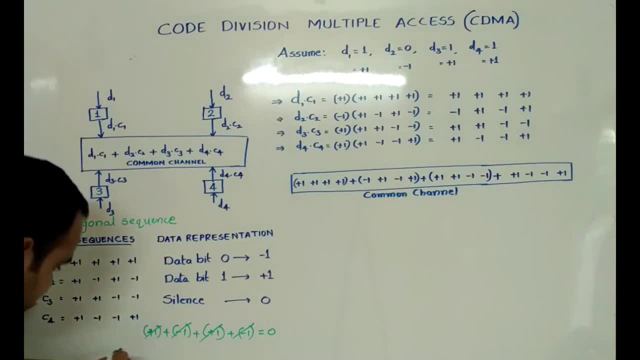 Assume that C1 or C2, C3, any type. So, for example, I am taking C3.. This one is C1 into C2, you will get 0.. Now I am taking C3 into C3. 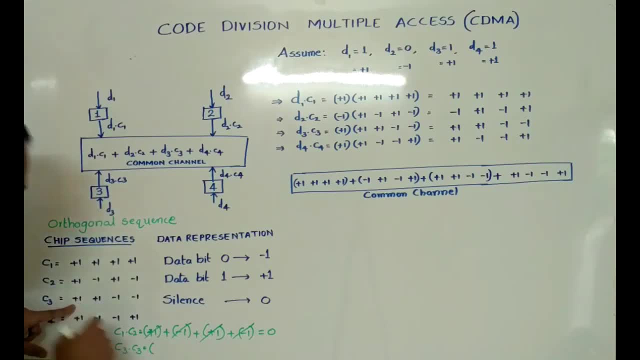 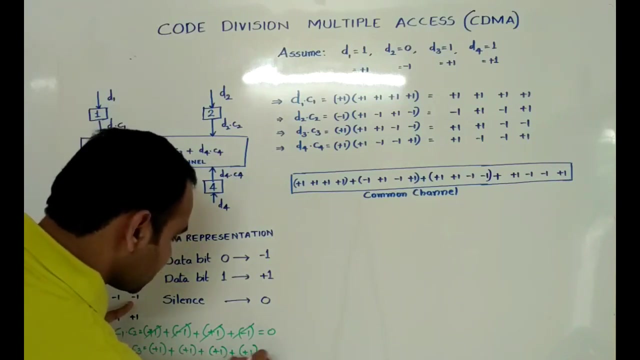 What happens is: Plus 1 into plus 1, plus 1.. Plus 1 into plus 1,, again plus 1.. Plus Minus 1 into minus 1, plus 1.. Minus into minus 1, plus 1.. 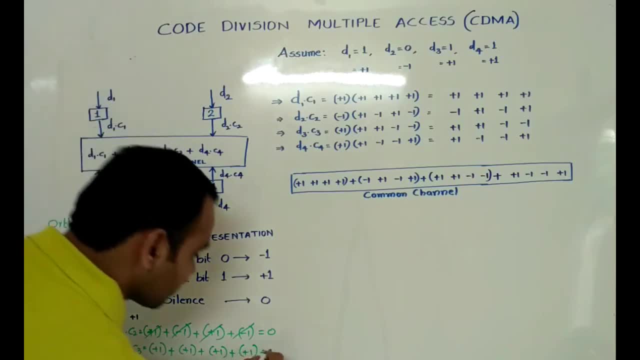 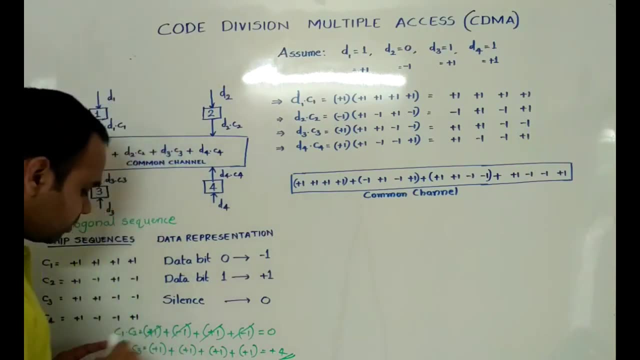 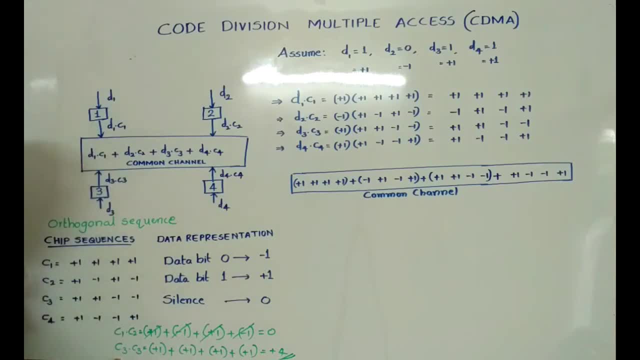 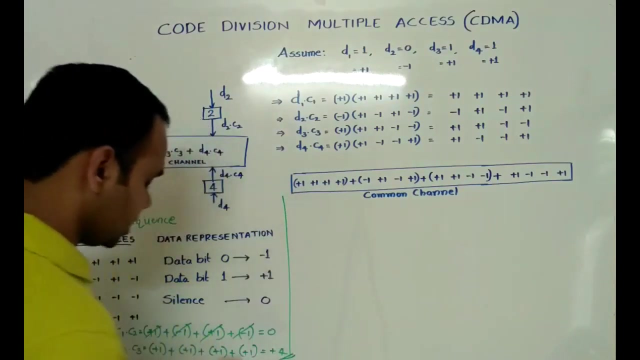 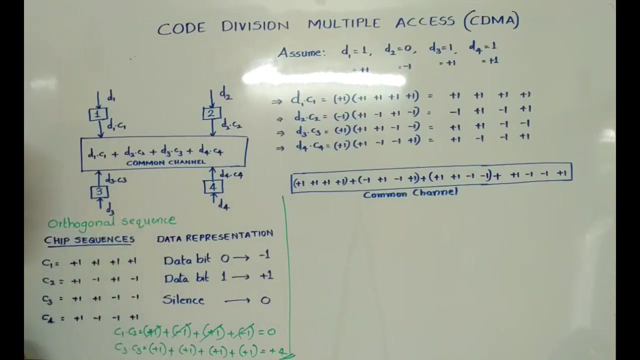 And if you multiply with any other code, then you will get 0. So this is actually very important logic. So by using this only, this entire communication is going to be successful. Okay, So now What we are doing is that those are the chip sequence, also called as orthogonal sequence, that I explained. 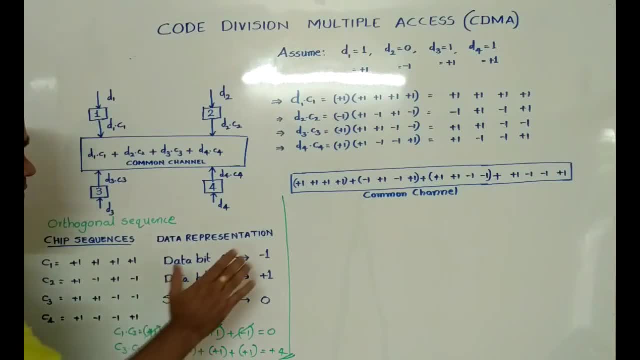 Now data representation. So data representation says that if any station wants to use, when they are sending, they may have the data like in terms of 0s and 1s, But here we are representing 0 as minus 1 and 1 as plus 1.. 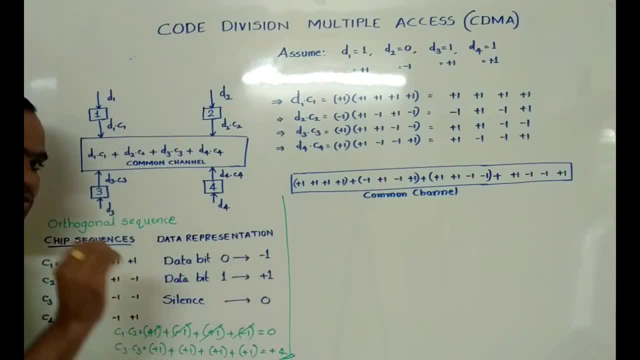 And if it is 0, that means that station is silent. That means it is not going to send any data, Okay. Otherwise, it is not going to put any data onto the channel. Okay, So now? So this is the scenario. 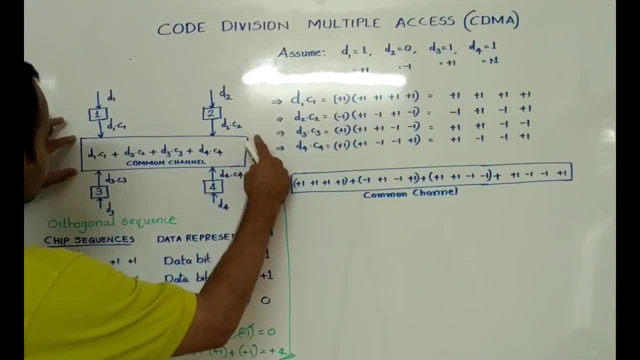 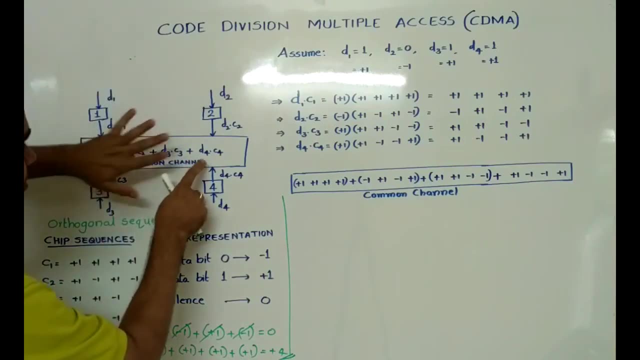 So the thing is that this channel contains some of all these datas: D1, C1 plus D2, C2 plus D3, C3 plus D4, C4.. Now assume that if any station wants to receive the data, assume that station 4 I am taking. 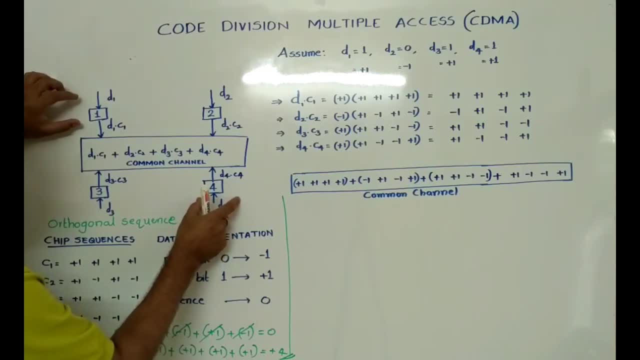 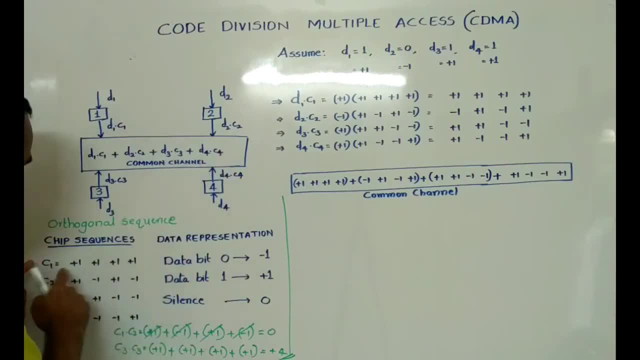 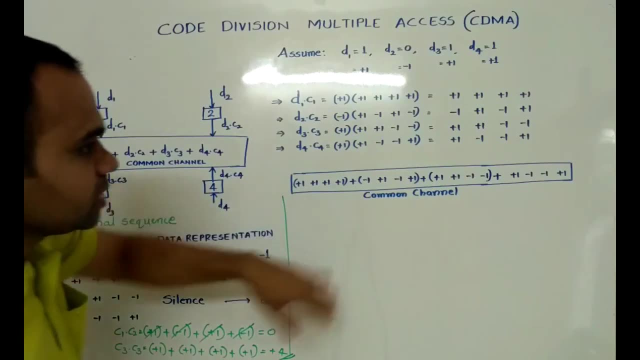 So if you multiply this entire data with C1, then what you will get is C1's data. you will get it. That means station 1's data you will get. Okay, I will be explaining here now soon. 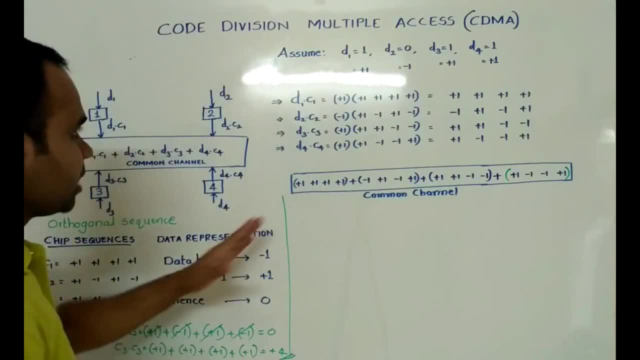 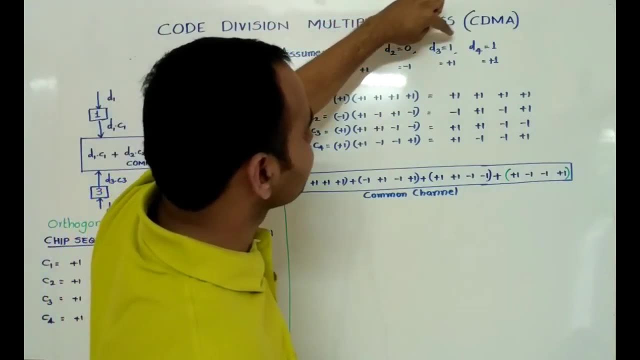 Okay, So what I have done here is- I took one example, That is, D1- C1.. Okay, D1's data is 1, D2's data is 0, D3's data is 1, D4's data is 1. 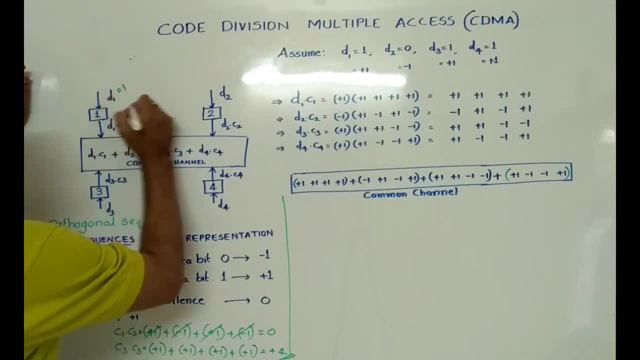 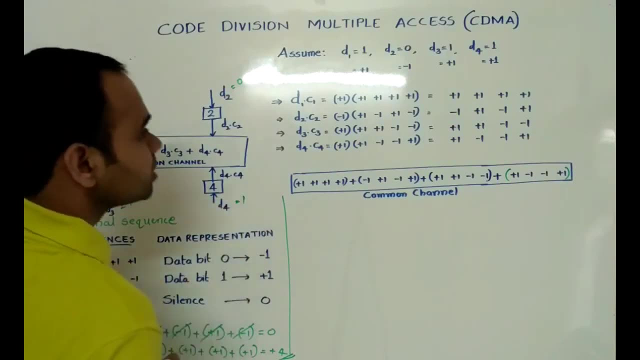 Okay, that means D1 wants to send data as 1, D2: 0, D3: 1, D4: 1. So according to this representation, data representation: If it is 0, we have to make it as minus 1. 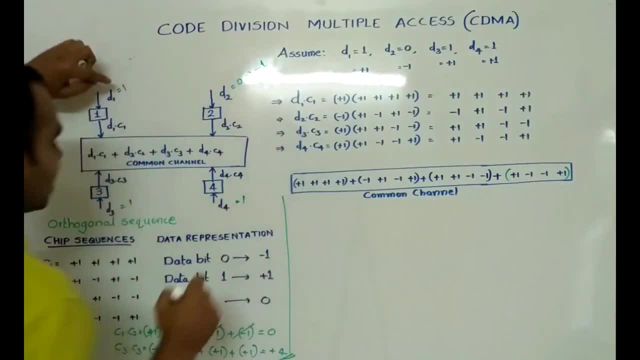 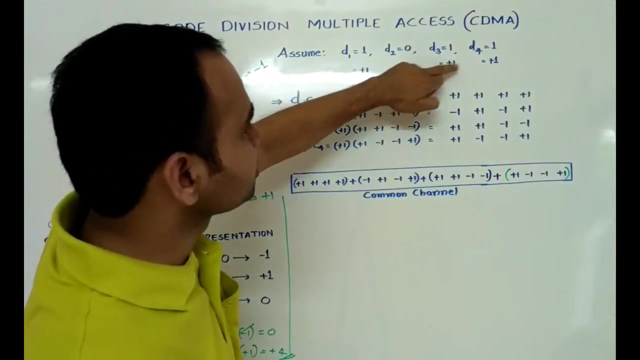 That means here it will become minus 1. 1 means plus 1, and this one also plus 1 and this one also plus 1. Okay, so that's why I meant as D1, 1 means plus 1, 0 means minus 1, 1 means plus 1, plus 1. 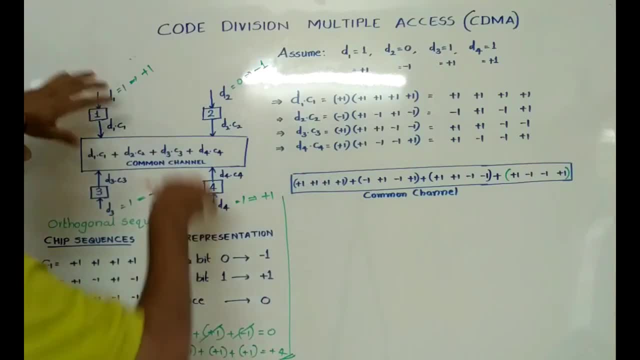 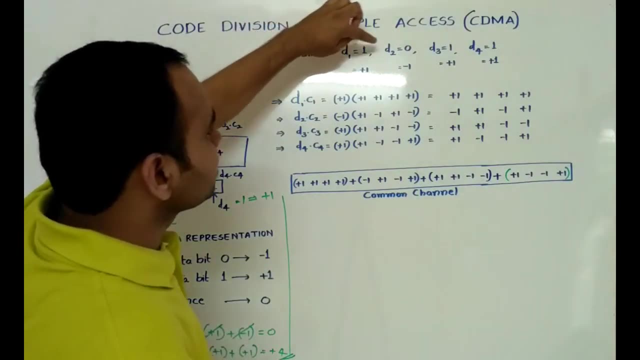 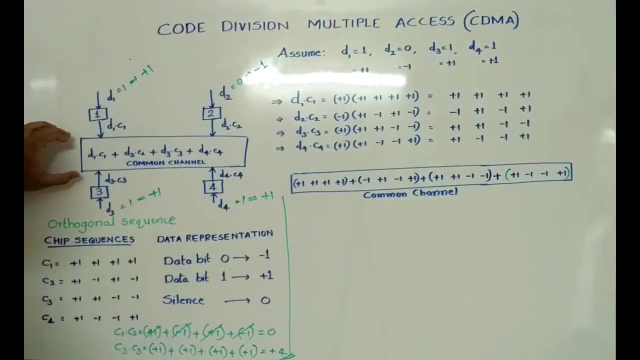 Okay, now assume that all stations are putting their data onto the channel. Okay for communication. So thing is that, see D1, D2. So D1, D2. Now station 1, station 1's, you know- put the data onto the channel as D1, multiplying its data with code 1. 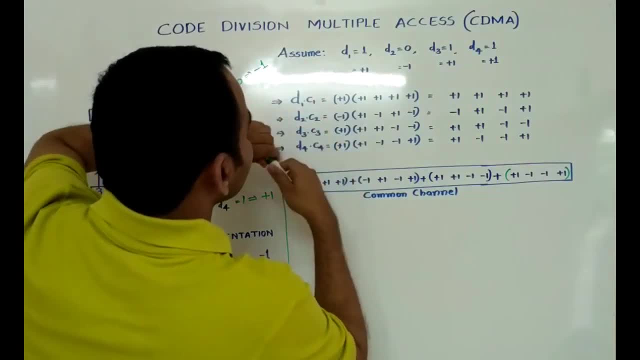 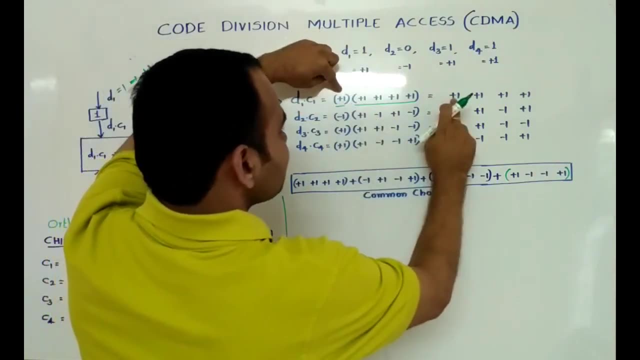 So D1, C1. What is D1?? D1 is plus 1, This D1 is plus 1 and this entire is C1. Okay, if you multiply this Plus 1 into plus 1, plus 1, Again plus 1 into plus 1, plus 1. 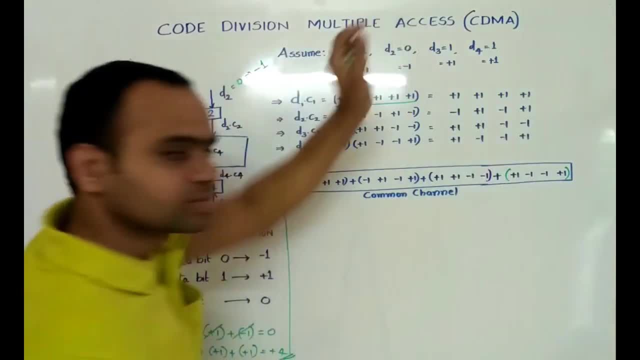 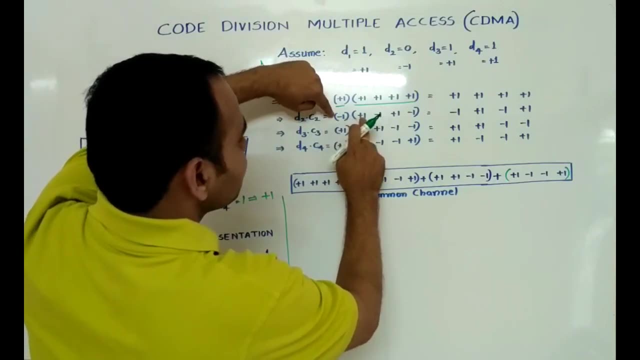 Plus 1 into plus 1, plus 1, Plus 1 into plus 1, plus 1. Okay, in the same way D2, C2. D2 is what Minus 1, Minus 1 into plus 1, minus 1. 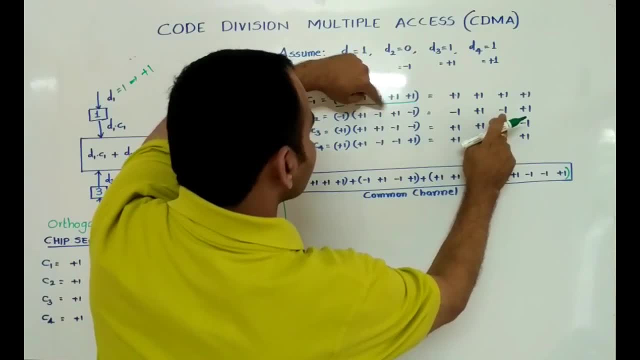 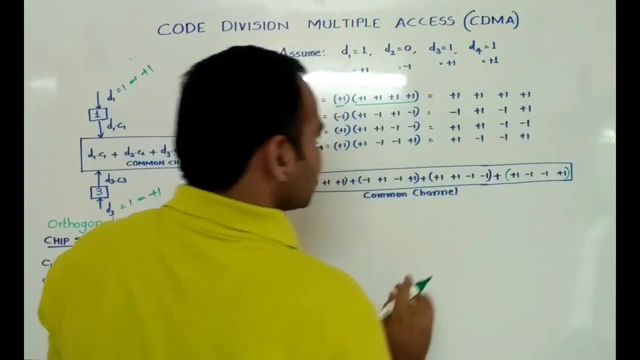 Minus 1 into minus 1, plus 1. Minus 1 into plus 1, minus 1. Minus 1 into minus 1, plus 1. Okay so D3, C3 and D4, C4. Okay, so I calculated here. 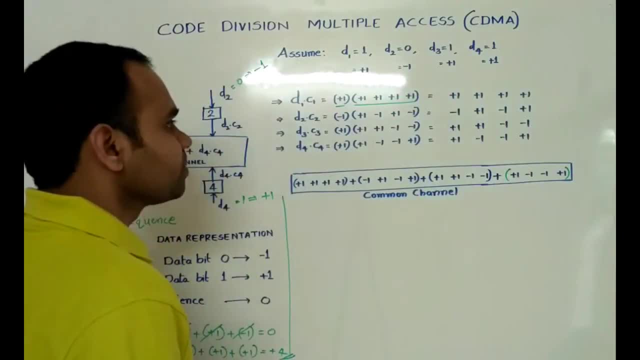 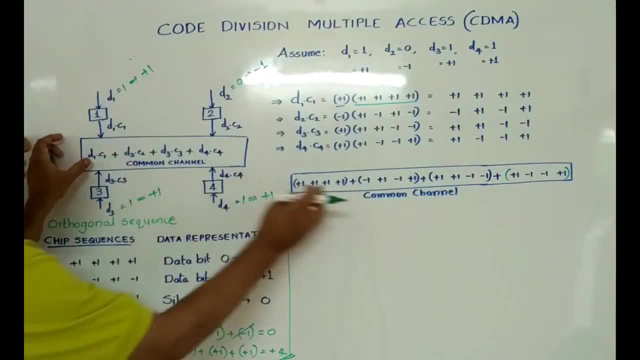 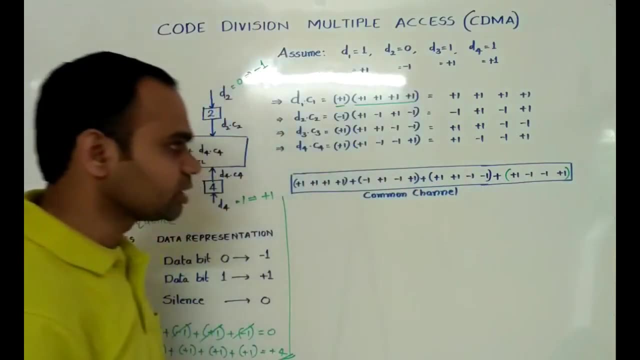 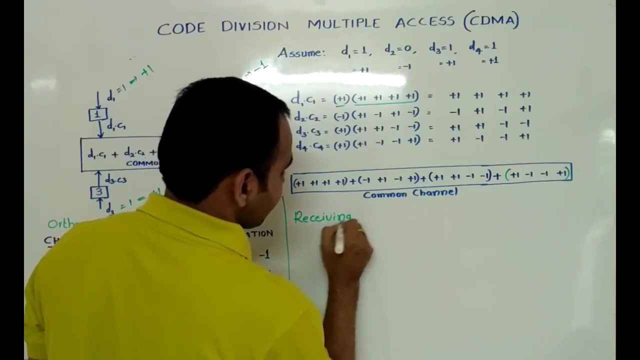 minus 1, like this: D1, C1, this one D2, C2. is this one? D3, C3. is this one? D4, C4. is this one? Okay, now at the receiving end, Now at receiving side. Okay, Now, if any station. 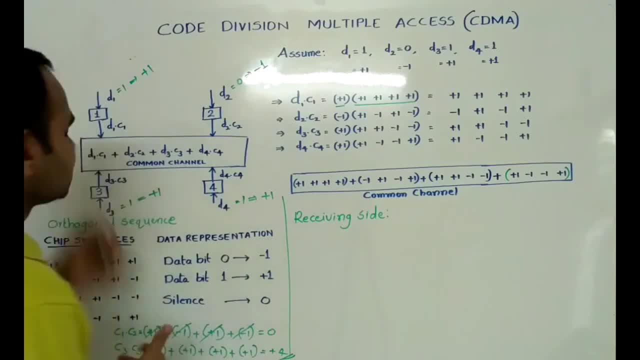 Assume that D3, like station 3 or station 4 or station 2 or station 1, Whatever you take. So if any station wants to receive any other station's data, Assume that if I want to receive station 2's data, What is station 2's data equal to? 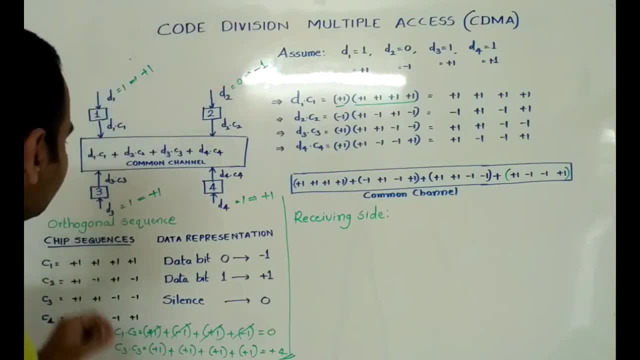 That is 0, So what I have to get, Minus 1. Okay, assume that now station 3- Station 3 is Station 3- wants to receive the station 2's data, Then what it does is, Whatever the data is there, It will be multiplying with the station 2's code. 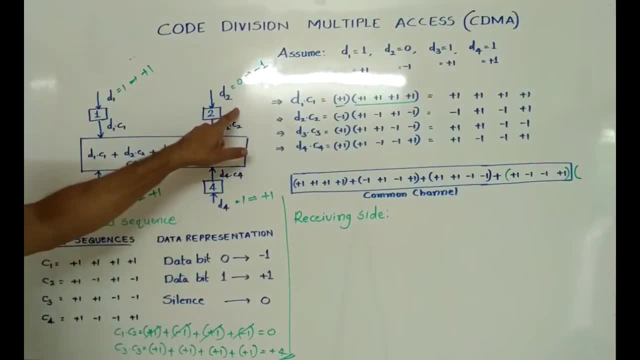 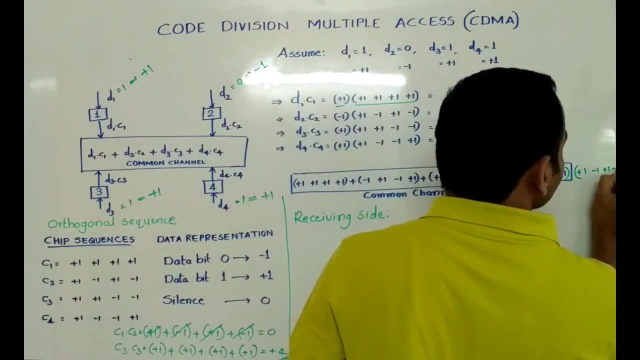 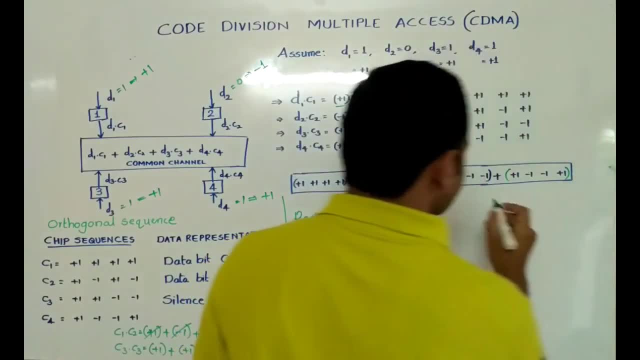 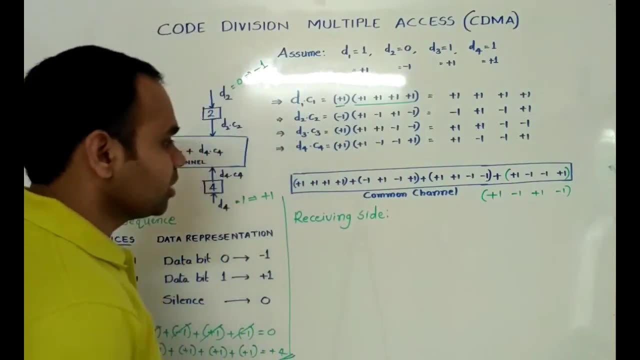 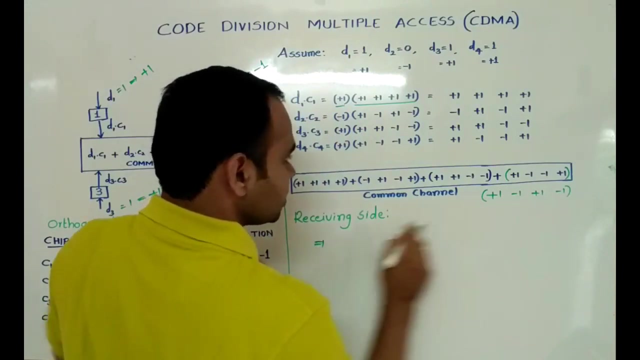 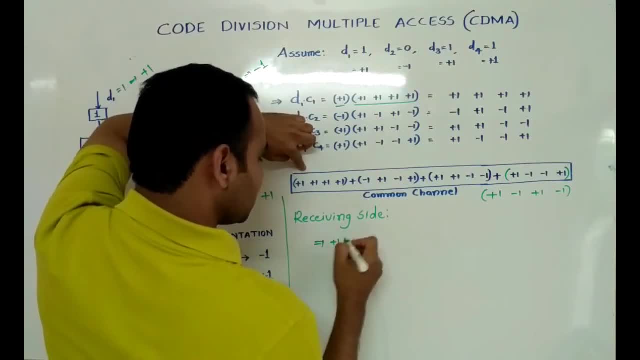 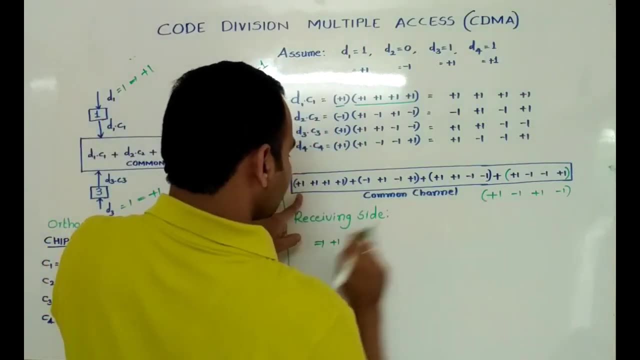 And I have to add all these things: Okay, plus 1. Okay and plus Or plus. anything is Plus into minus, minus, only So directly I am writing: So plus 1 into plus 1, plus 1, Plus 1 into minus 1, minus 1. 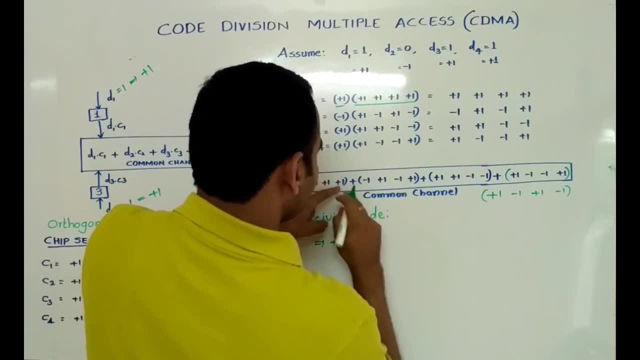 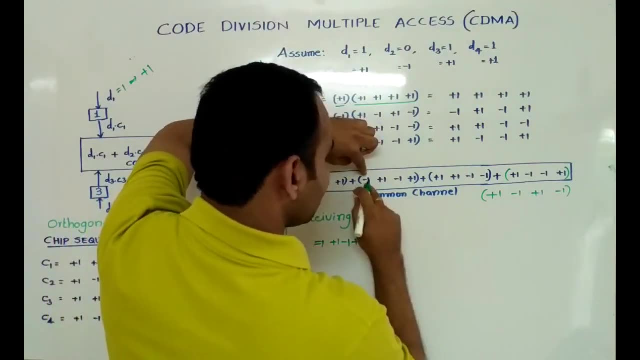 Again plus 1 into plus 1, plus 1 And plus 1 into minus 1, minus 1. Okay, Again, plus Minus 1 into plus 1, minus 1, Plus 1 into minus 1, minus 1. 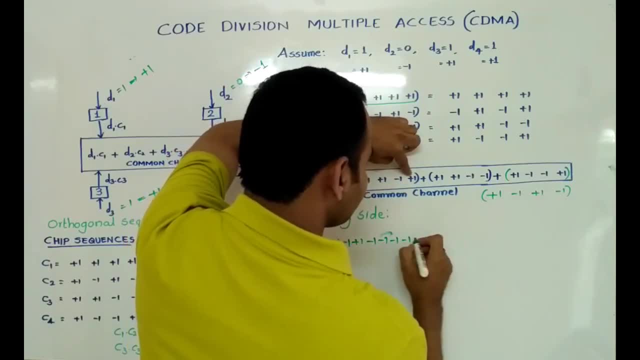 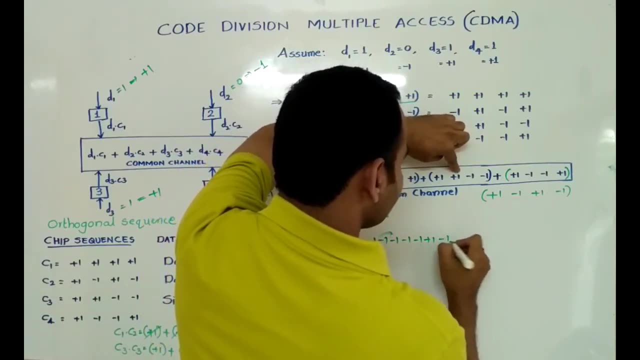 Minus 1 into plus 1, minus 1. Plus 1 into minus 1, minus 1, And again this one, Now plus 1 into plus 1, plus 1 Plus 1 into minus 1, minus 1. 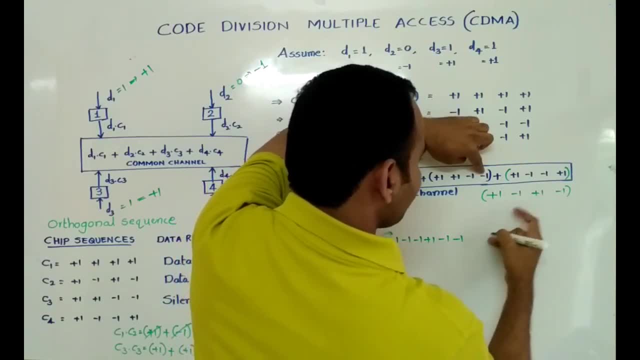 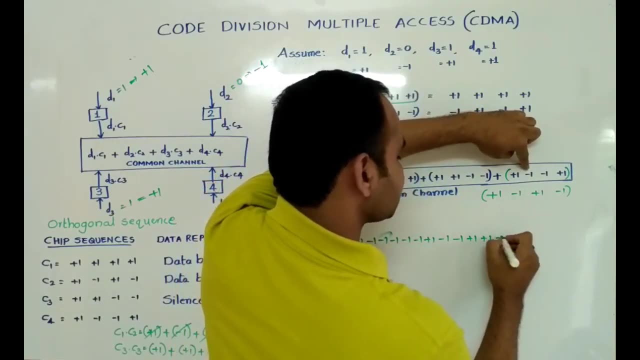 Minus 1 into plus 1, minus 1. Minus 1 into plus 1, plus 1, And again plus 1 into plus 1, plus 1. Minus 1 into minus 1, plus 1. Minus into plus 1, minus 1. 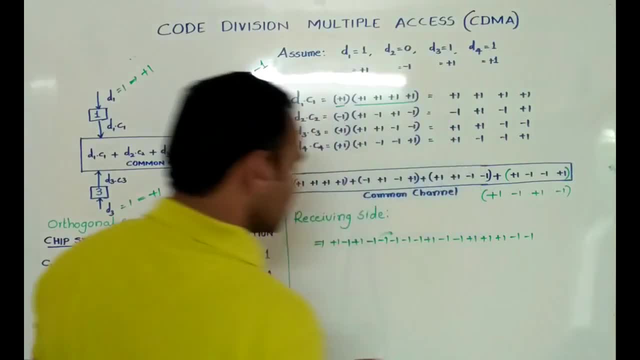 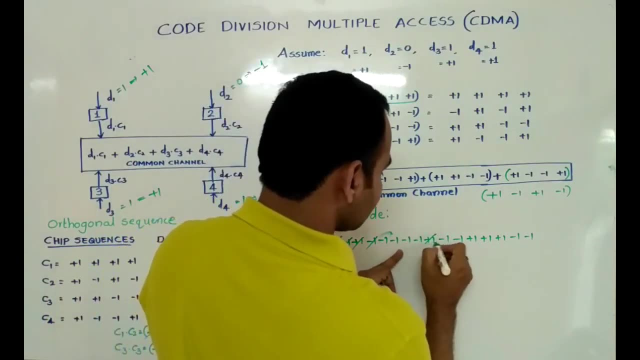 And minus Plus 1 into minus 1, minus 1. Okay, So now Plus 1, minus 1, Plus 1, minus 1. Cancel Minus 1, minus 1, minus 1. See Plus 1, minus 1. 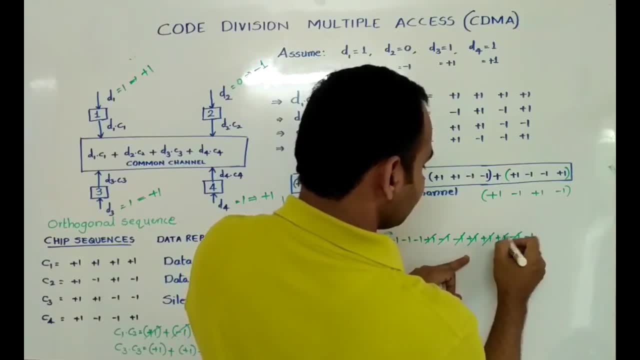 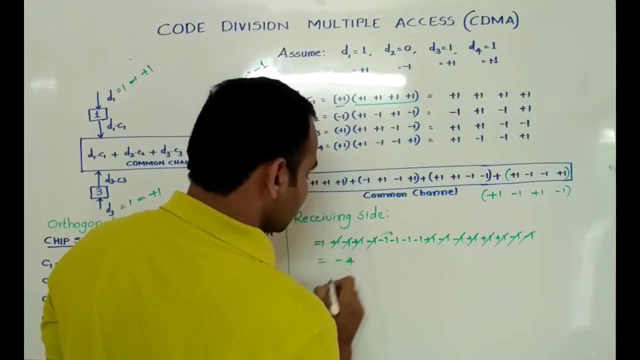 Again: minus 1, plus 1, Plus 1, minus 1, plus 1, minus 1. What we got? Minus 1, minus 1, minus 1, That means minus 4. So we got minus 4. 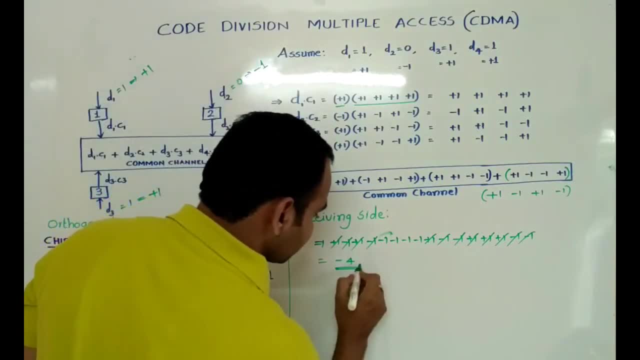 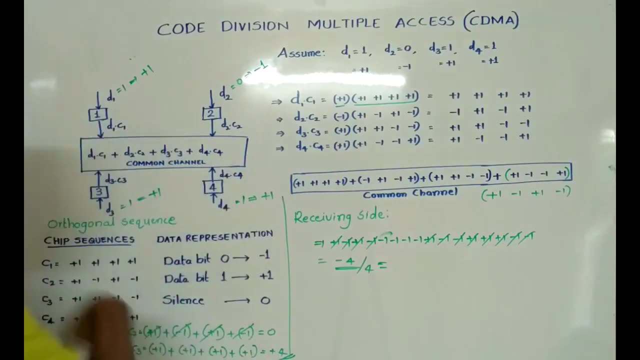 The thing is that We have to divide this minus 4 by 4 To get the actual value. So why we are dividing by 4 means There are 4 stations. That's why we have to divide by 4. Okay, So what we got is minus 1. 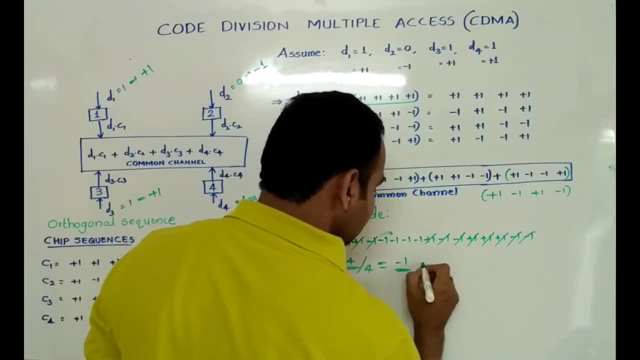 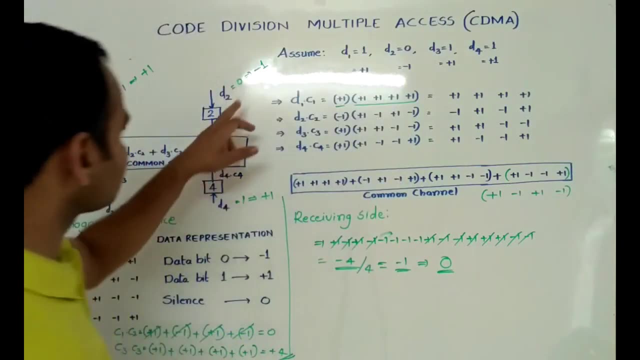 So what is minus 1? actually, Minus 1 is representation for 0. Minus 1 is representation for 0. So now we got station 2's data. What is station 2's data? That is 0. Okay, So in this way we are going to get the data. 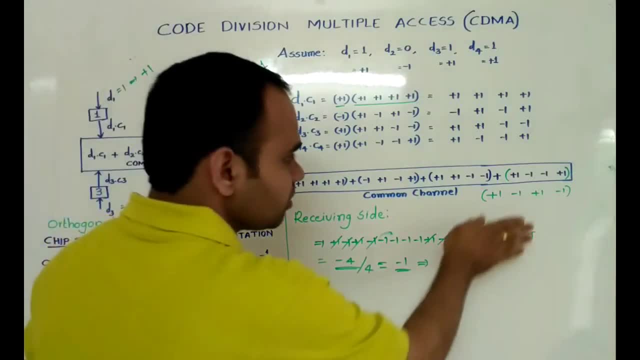 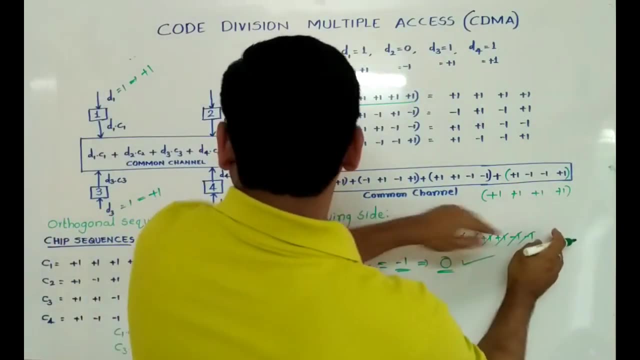 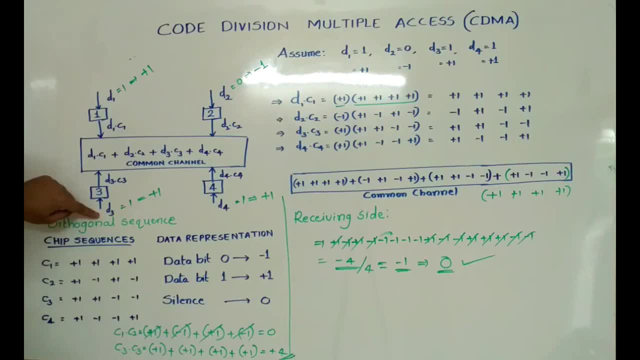 If you want to receive station 3's data, Then what you have to do is You have to multiply with station 3's code. Okay, So by using this code You will get, If you multiply this entire channel data With code, With this station 3's code. 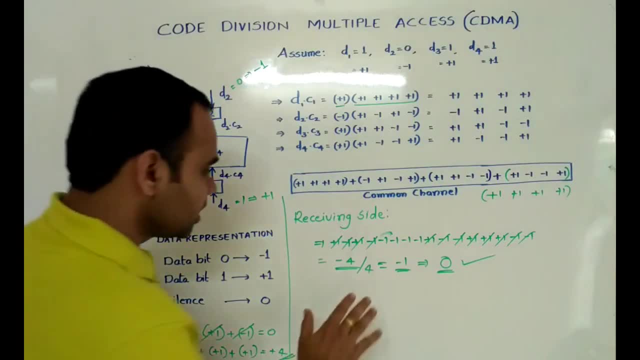 You will receive station 3's data. Okay, In this way it is going to be. You know happened.